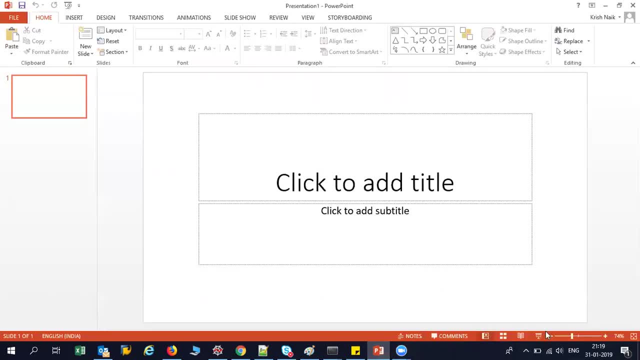 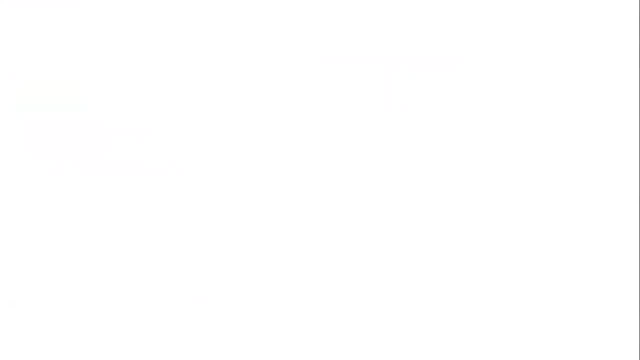 learning problem use case. To begin with, what I will do is that I will just open a blank space If you have not gone through the simple linear regression. I have provided the link in the description of simple linear regression. Please go through that video first. 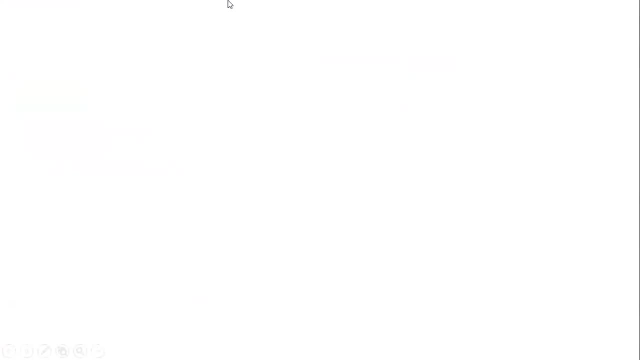 before going into it: Usually simple linear regression. when we consider a simple linear regression, it is basically given by. I will just write it down and we will try to compare. what is simple linear regression? How is it different with respect to multiple linear regression? I will write it down over. 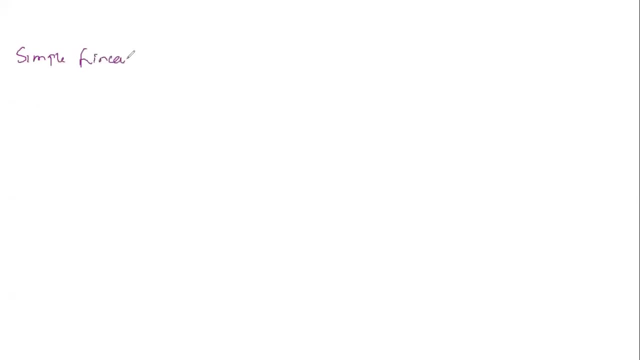 here as simple linear regression. Sorry for my bad handwriting, but just try to understand this. I will just take red color. Now suppose if I have a scenario where my x-axis is basically, you know, size of house and my y-axis is basically the price of the house In simple linear regression. 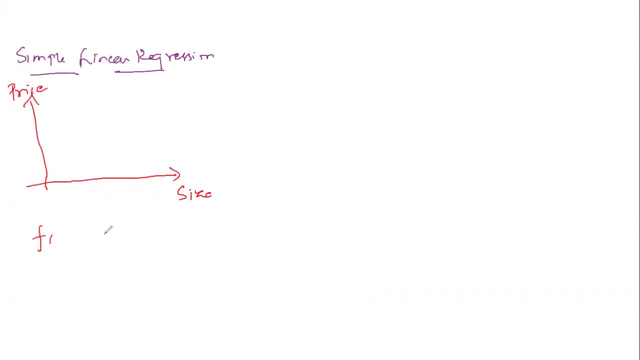 we basically be having two features. One is F1, one is F2.. This F1 is basically the size and this F2 is basically the price. F1 becomes my independent feature. F2 becomes my dependent feature Based on this feature. as we know that usually, whenever the size 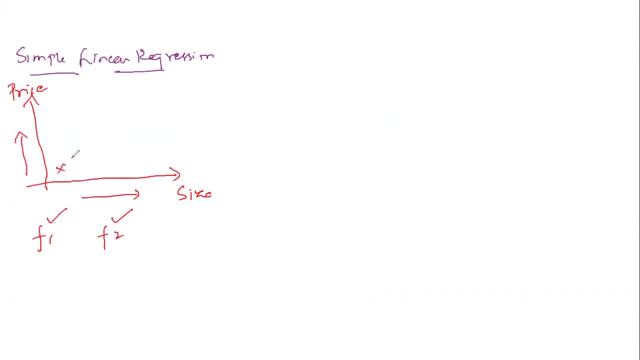 increases, the price also increases. Suppose, if I scatter some of the point, something like this: This is just randomly taken, guys. What we will do is that, in simple linear regression, we try to find a balance. This is a point. This is a point. This is a point. This is. 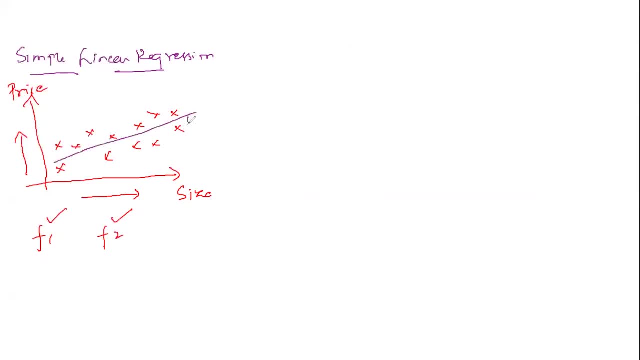 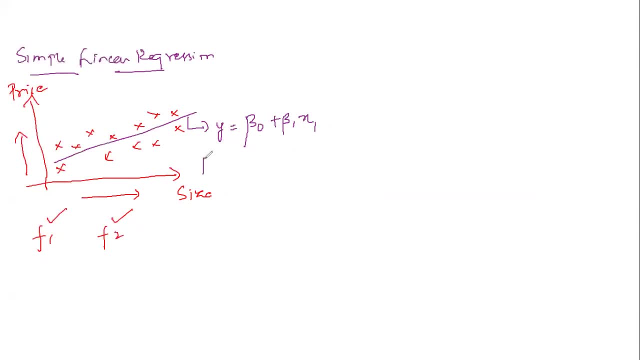 x1 as my size. how will this equation get converted to? It will get converted to. price is equal to beta 0 plus beta 1 into size, As we know that beta 0 is equal to between visiting the house to find something and two people are Muttering toendes. Similarly, if 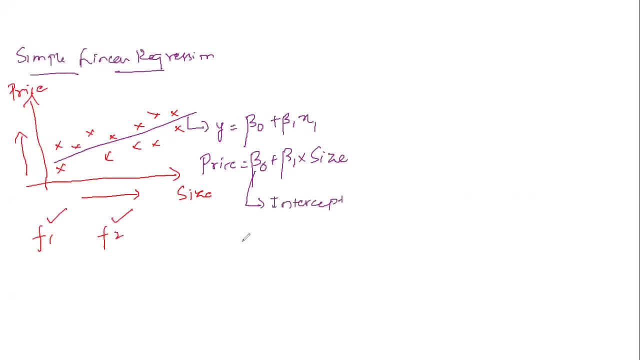 we look at the commercial model of 구리 시리, наша 시. vector is also function of type, the intercept and beta 1. beta 1 is basically my slope slope or coefficients. coefficients, now, when we are discussing about this equation, this intercepts basically indicate that when my size is 0, what will be my base price? so this is. 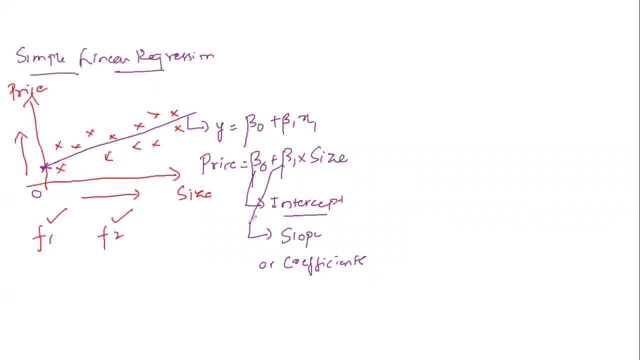 the value of my intercept in that particular best fit line and slope basically indicates that with the unit increase in size, what is the unit increase? the slope, that is what this particular value is actually specified by this particular slope value. okay, so beta 1 is nothing but slope, or? 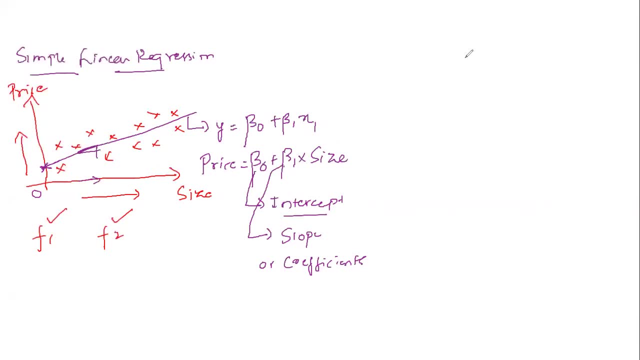 coefficients. now, how is it different when compared to multiple linear regression? okay, now, when I compare multiple linear regression, this basically indicates that now I have, I will be having many features. it will not be just one expression, will be present, we'll be having other features also. suppose now I have f1, f2. 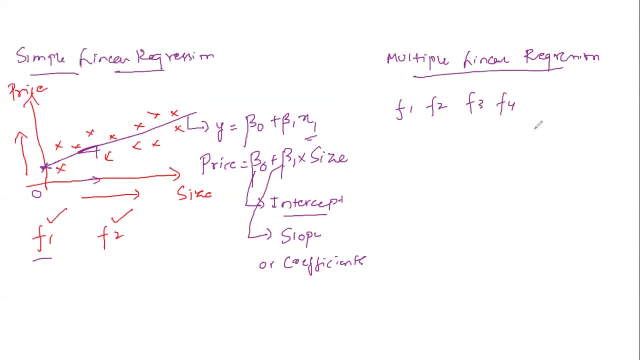 f3, f4 features, and my output feature is basically my f5 feature. now suppose I'll take the same example. suppose my f1 is science, my f2 is number of bedrooms. right, then my f3 feature can be locality- locality of where the house is present. 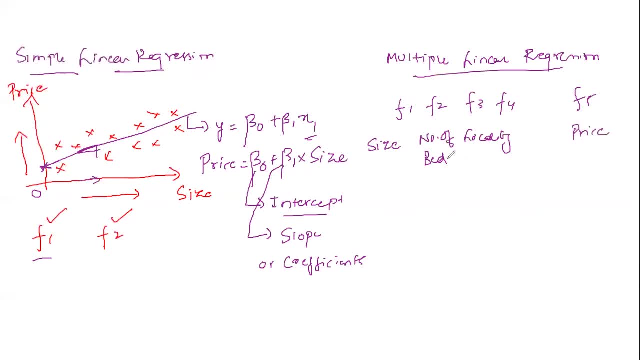 and f4 may be some other feature, and f5 is basically my price. so now you can see that multiple independent features can also impact the price. now, when I'm discussing about multiple linear regression, now my this equation, when I'm trying, when I have this equation, will basically get converted to something. 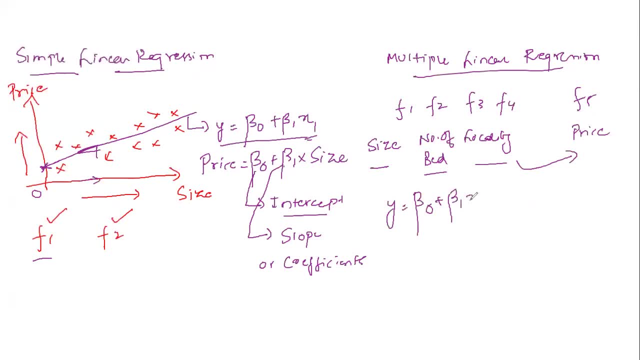 like Y is equal to beta 0 plus beta 1, X, 1. X 1 is basically my size feature, beta 2 into X 2. now X 2 will become number of bedrooms right now. similarly, I'll have beta 3 into locality, which will be my X 3, and this Y will basically be my price. 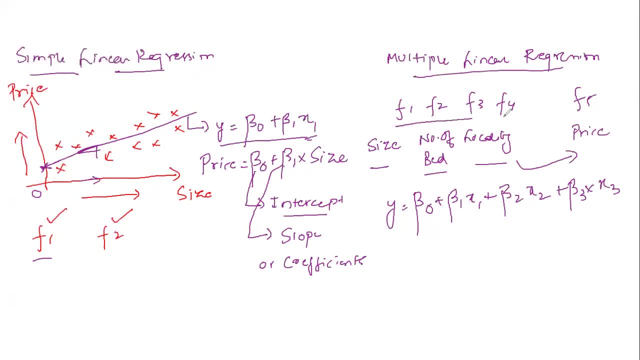 now, whenever I consider multiple independent features and when I have one dependent feature and if this is a regression problem, I basically call this as a multiple linear regression, and this is how my equation gets changes. now, our aim in multiple linear regression is that we need to compute beta 0, so beta 0. 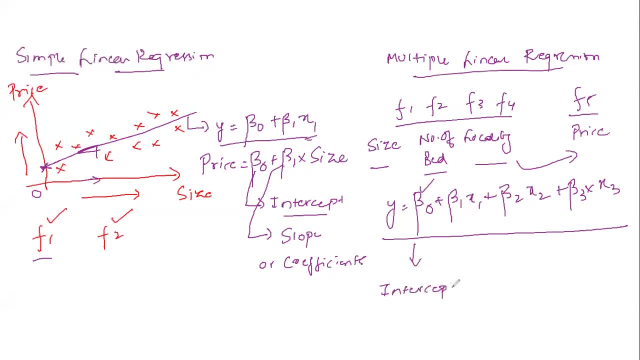 is again the intercept. again the intercept. beta 1, beta 2, beta 3 are the slopes of the coefficient with respect to this independent features. now that basically indicates that if I increase the value of X 1 by 1 unit, then this beta 1 says that by how much value? 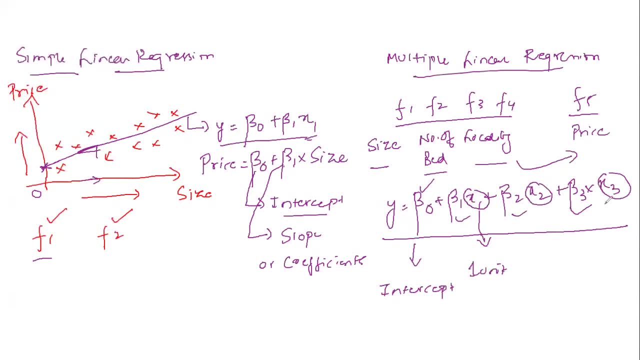 it will affect in the price. similarly, with respect to beta 2 and beta 3- and this is a small theoretical description about multiple linear regression- we will be using the same sklearn linear regression library- linear regression library to solve this problem. now let us go ahead and see a use case where I will be having a use case I'll be having 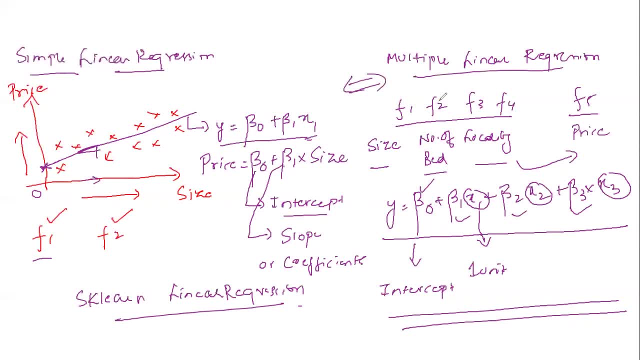 a data set which will be of multiple linear regression type, where I'll be having multiple independent features and I'll try to find out the output value. yes, now let's go ahead and understand the practical part. now, here it is. what I will do is that I'm going to 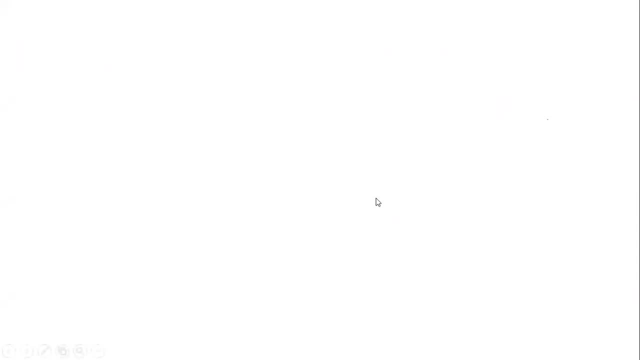 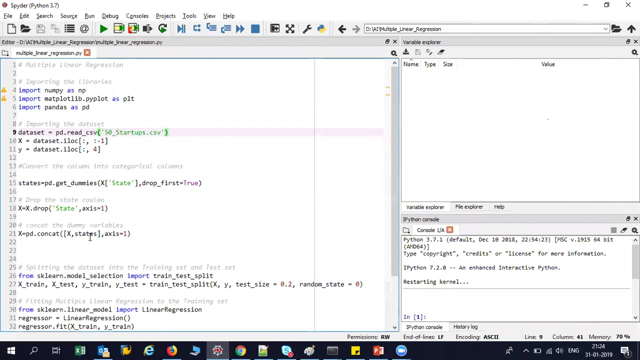 use that. I will try to open my spider ID. I'm going to use spider ID for this purpose. this is my spider ID. make sure again, guys, this code, the data sets, the data set, which will be in the CSV format, will be uploaded with the github and that github link is provided. 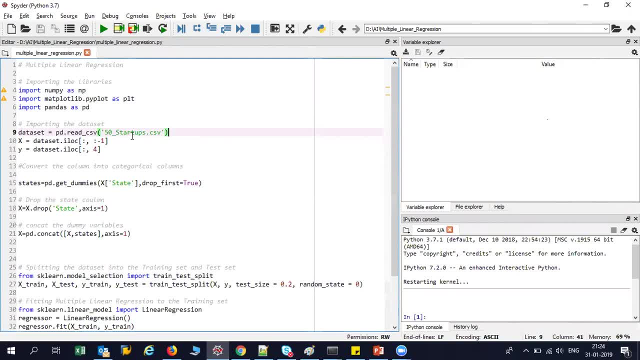 in the description box. first of all, I have a data set which is called as 50 underscore startups dot CSV. I'll tell you about this particular data set. first, let us let us all import this data set, and then I will go ahead and import this data set and then I will go. 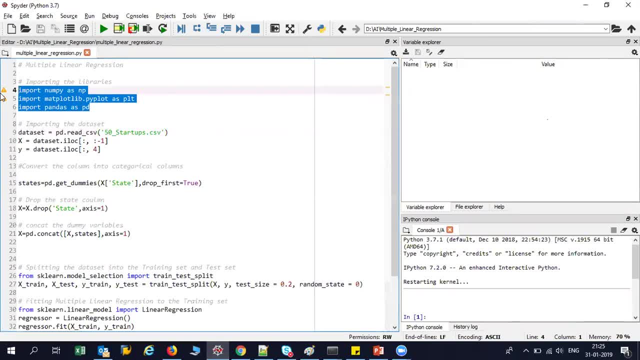 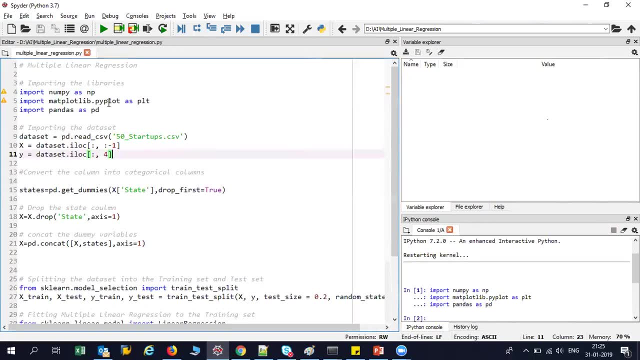 ahead and import this data set and then I will go ahead and import this data set and then it goes to this library. I'm importing NEM pi, mat plot libran pandas. you know that NEM pi is basically used for getting People read the function and that matplotlib is basically used for visualization. ponder this basically. 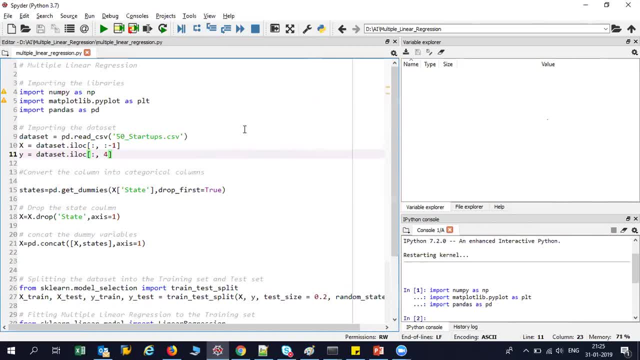 used for leading the. it is a first step. I am going to lead my insight. so my data set is in this particular location, only in my working space directory that we can see over here. and make sure you also set up the working space director. output your CSV file there. that, Wow, I'm reading this 50. 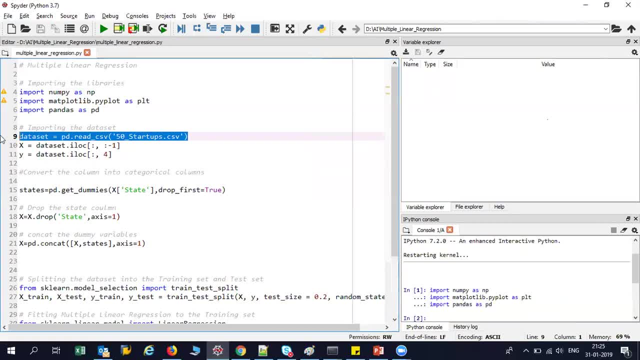 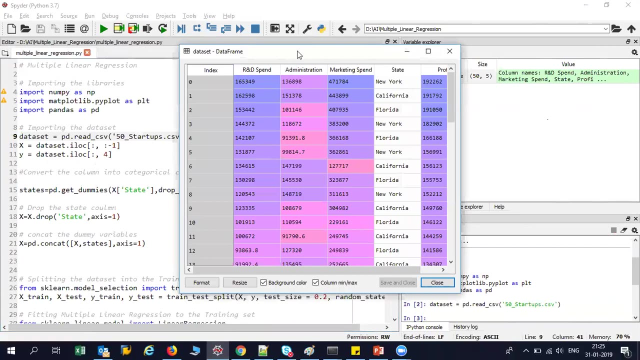 startupscsv. now, as soon as i read it, i'll just explain you about this data set and what this data set is about. so it will take some time for execution because it is a huge data set- not a huge data set, but due to some interesting time, let me double click this data set. now, here you 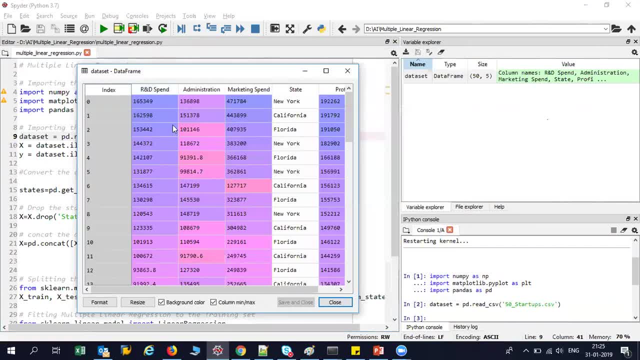 can see that my data set basically has. so this is the information of 50 startups in various states. okay, have features like r&d, spend administration, marketing, spend state and profit now in this. if you know that just by seeing this particular data, profit is basically my 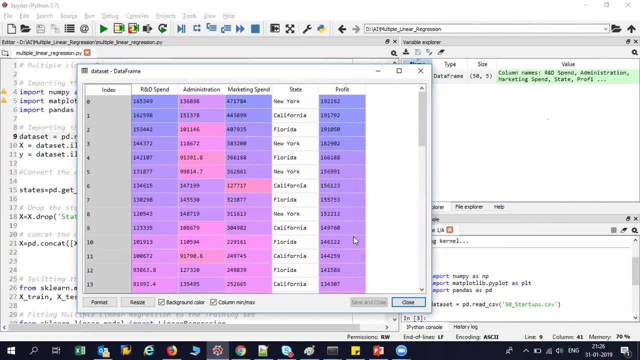 dependent feature. now what this use case is all about, i have to find out profit based on this feature on r&d spend. so basically, a company has invested some amount of money in r&d, some amount of money in administration and some amount of money in market. 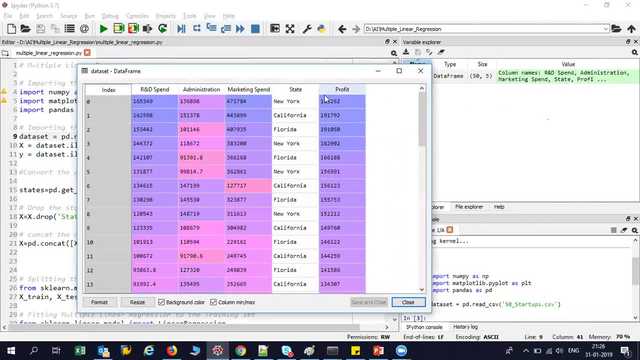 from this many states so, and this was the total profit that they were able to make it. right now our aim should be that, by getting the values of r&d spend, administration, marketing spend, and from which state, i should be able to predict what is the profit value. so this is a kind of regression. 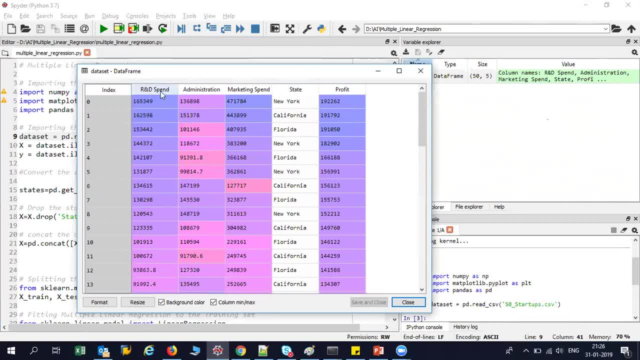 problem and just by seeing the data set, it looks like this: all are independent features that i have: r&d spend, administration spend, marketing spend and state are my independent features, whereas profit is my dependent feature. so always whenever we load a data set, our first work is to divide into dependent and independent features. so for 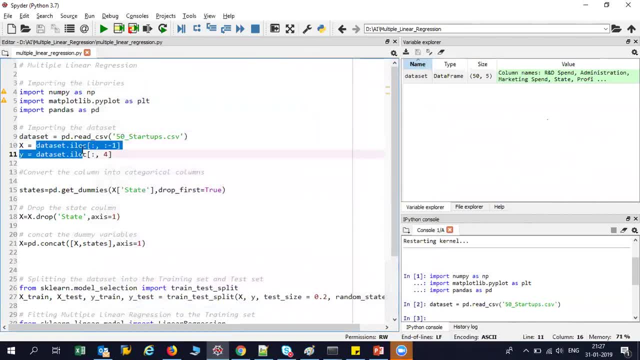 that i've written a code where i'm taking data set dot, i log, colon, comma, colon minus one. this basically indicates that, except from the last column, the last column is basically my profit column. except from the last column, i'm going to take all the columns and store it in my x. 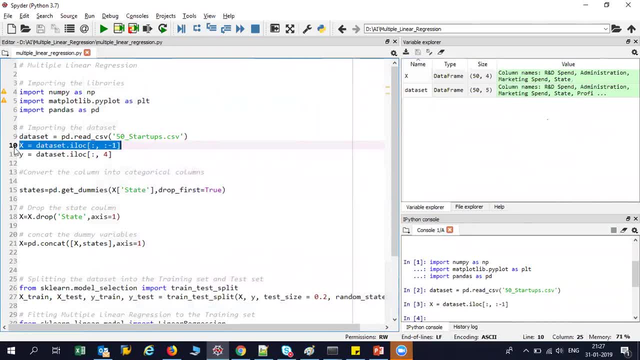 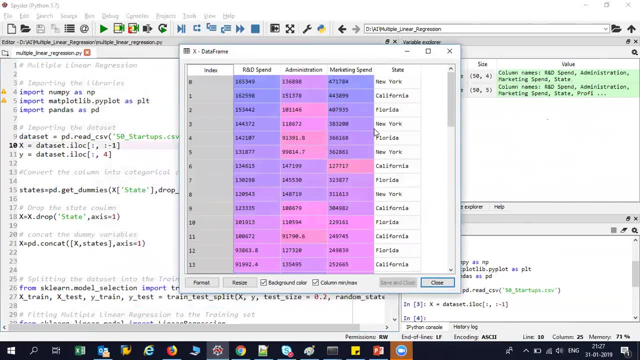 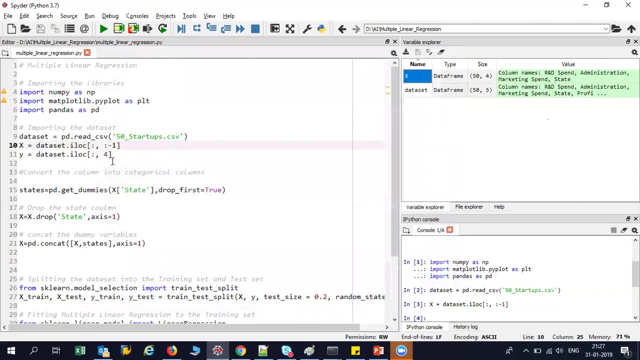 variable and this x variable is nothing but independent feature. just execute it. It has got executed perfectly. You can go and see your X dataset. This is what you have Now. the next thing is that we will try to, you know, create our dependent dataset. Now, dependent dataset is basically given my datasetilog. 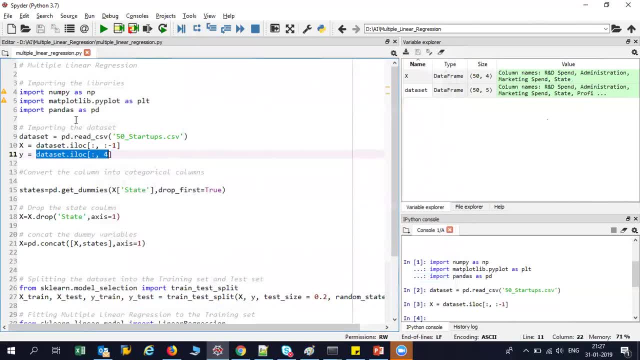 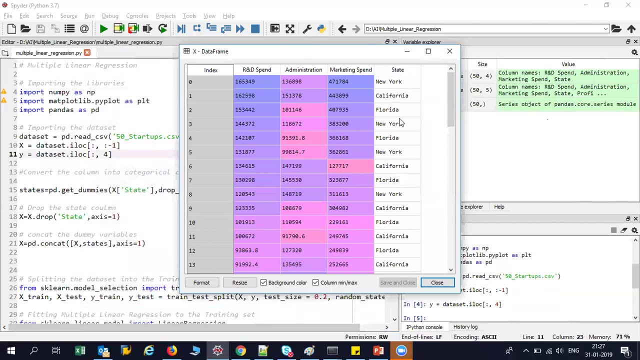 colon, comma four. The fourth location is basically my profit, So I'll also execute. So Y will basically be having my dependent dataset, whereas X will be having my independent dataset. Now the next thing is that if I go and see on my dataset, I have a state column and this looks like a category column, right We. 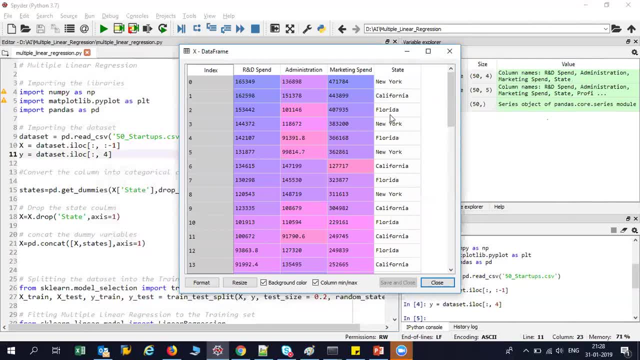 have three unique categories and every time we'll be having three unique categories. One is New York, one is California, one is Florida. We have to convert this category feature into one hot encoding. If we had just two categories at that time, we could convert that into label encoding. right Now we 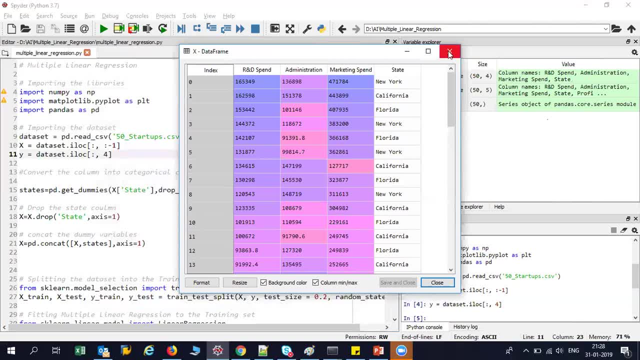 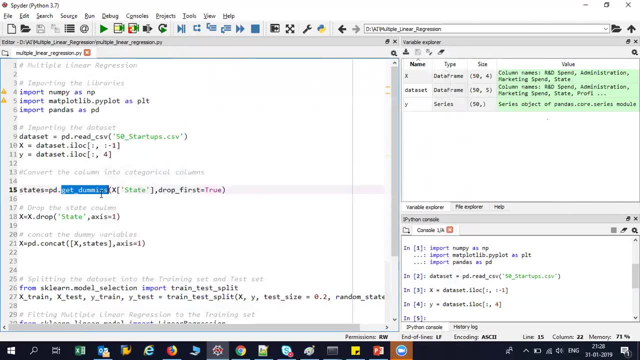 have to convert this into one hot encoding. In order to convert this into one hot encoding, we have to convert this into one hot encoding. So we have to convert this into one hot encoding. I'll be using a function inside pandas, that is, get underscore dummies. Get underscore dummies helps you to create dummy variables with. 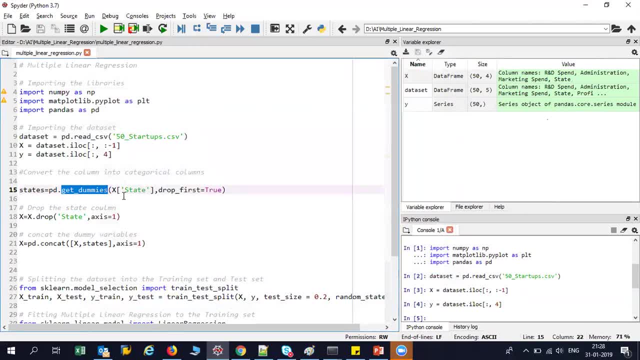 respect to the number of categories that are present Inside this. I am using the X state value. So basically, in my X feature, which is my independent feature, I'm taking the state and I'm converting this into dummy variables And make sure you 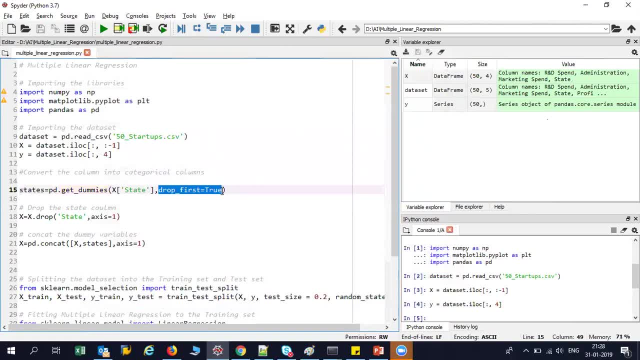 include this drop underscore first is equal to two. That basically means that once my, once my, once my data set, once my category feature right Once it is converted into three columns. suppose I have New York as one column, California as one column. 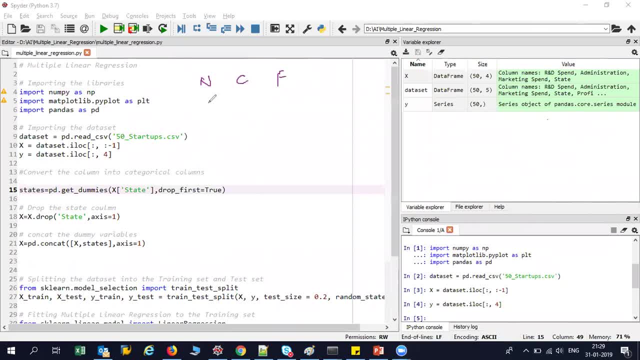 and Florida as one column right. So whenever there will be a data of New York, my value will become one zero zero. And whenever there will be a value of California, it will become zero, one zero. And whenever we have Florida, it will. 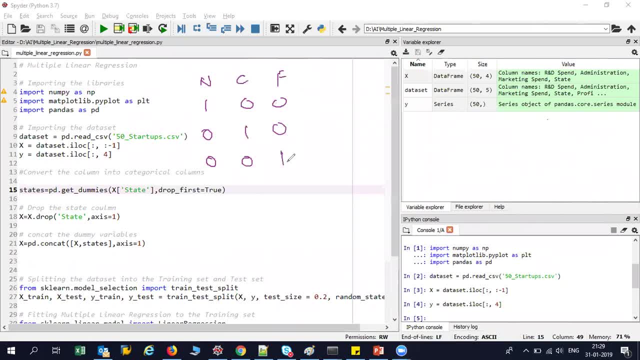 become zero, zero one, And this actually helps you to indicate that which column, which column we are referring to or which state we are referring to. But I think you can see over here, instead of taking all these columns, I can just take. 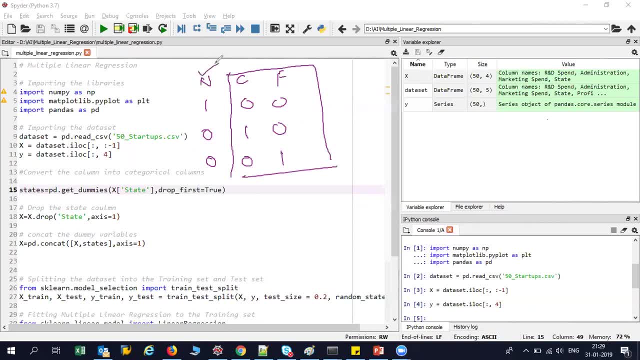 this two column and I can also indicate my New York feature in this. How See, whenever California we are talking about, then it becomes one zero. Whenever Florida we are talking about, it becomes zero one. But whenever we talk about New York, it becomes both zeros. 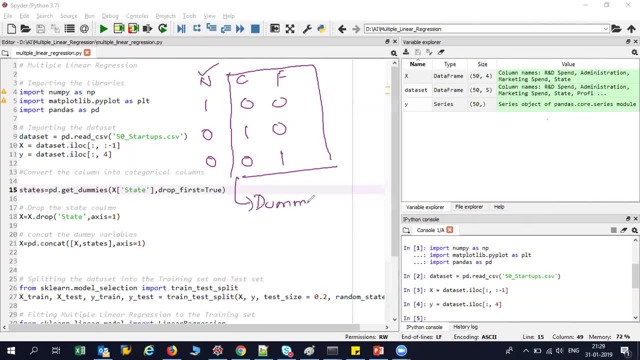 So this type of situation is basically called a dummy variable trap, Dummy variable trap. So we should always take care of this dummy variable trap And whenever we are converting our category features into one hot encoding or dummy variables. So this is how, as soon, 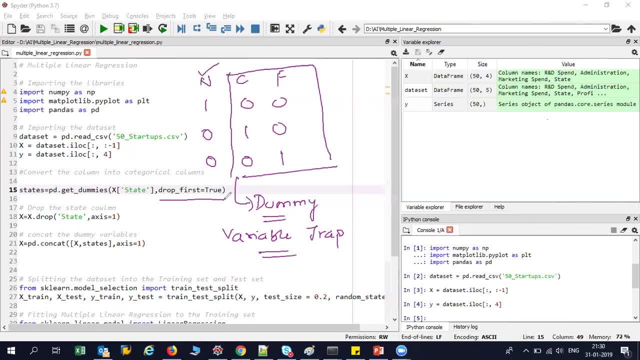 as I create. I have to just provide this: drop underscore first is equal to true, right? So drop underscore first is equal to true. What it does is that it removes the first column after dividing into one hot encoded values or dummy variables. right, I hope everybody. 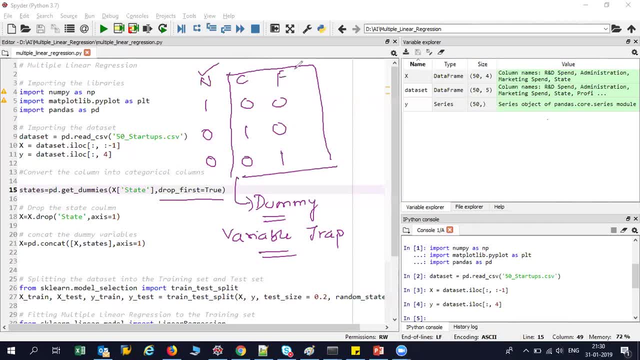 is understanding this. So this actually creates me a new data framework. In this data framework, I have two columns, So in this state's value, I'll be having two columns. Now let us just go ahead and understand more things. Now I'll just execute this and 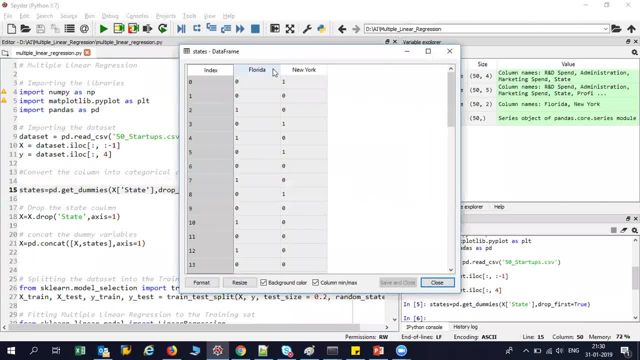 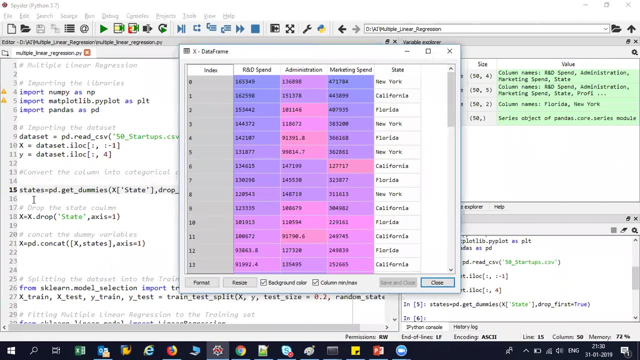 soon as it is executed. now you can see that I'm having a state column and I have Florida and New York. So California column is deleted. And what we'll do next? next, what we'll do is that still in my X I have the state. right Now this state has been converted into catalyzed. 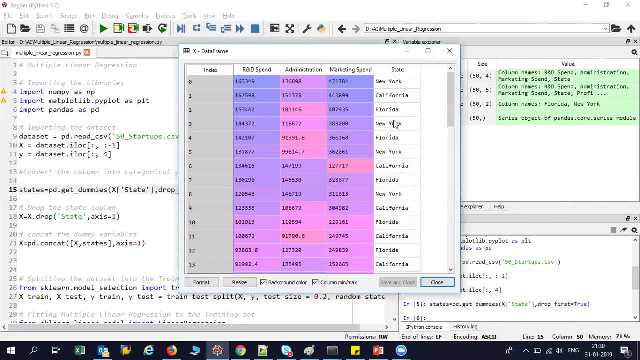 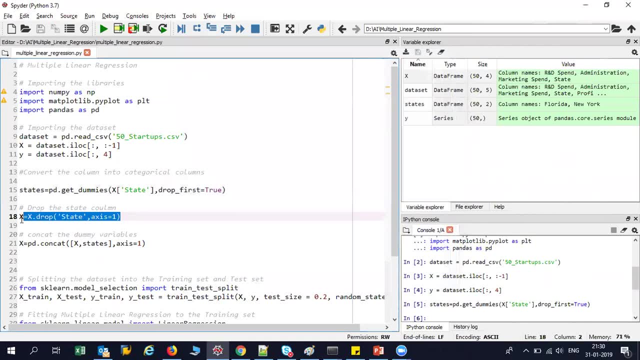 variables that is stored in this states variable right. So I do not require the state column anymore. So what I can do is that I can drop the state columns. So in this particular code I'm dropping the state column and I'm setting the access value as one, because the access 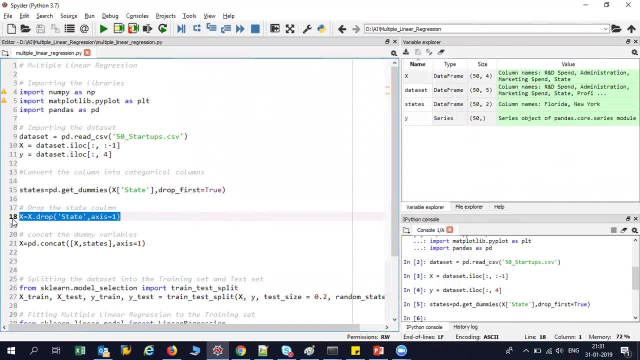 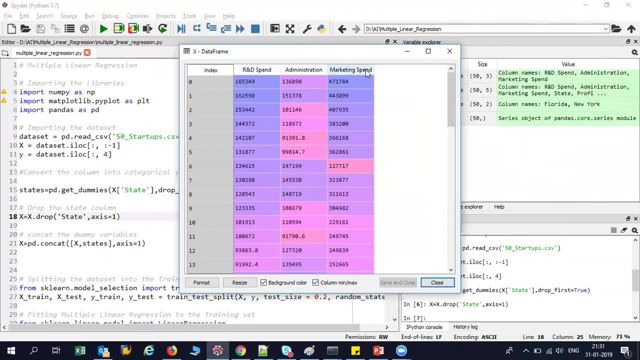 value one is equal to one actually saves us the column values. I'll execute this Now. you can go and see my X value. I have R and D spend, administration marketing spend. This is the process of all the data processing work that we are doing Now. the next thing is that 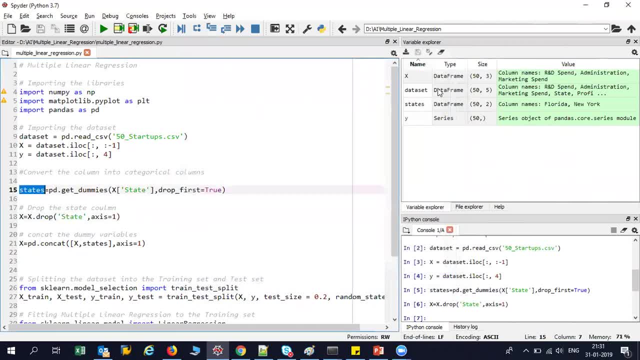 after dropping it, the state variables that were created, which are my dummy variables, has to be concatenated with this X variable. For that I'll be using pdconcat, And in that my first parameter will basically be X and states, which will be provided in the list. 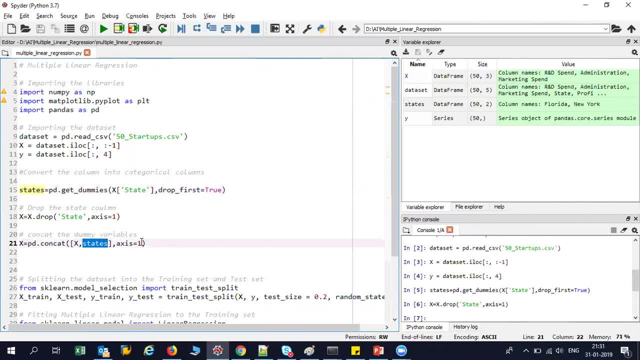 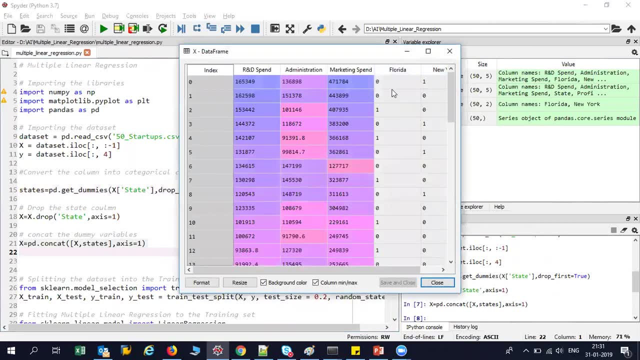 So both of this I'm doing, the concatenation of the data frame, And again, the access value should be one. So as soon as I execute this now, you can see that my X variable, if I go and see, is having. 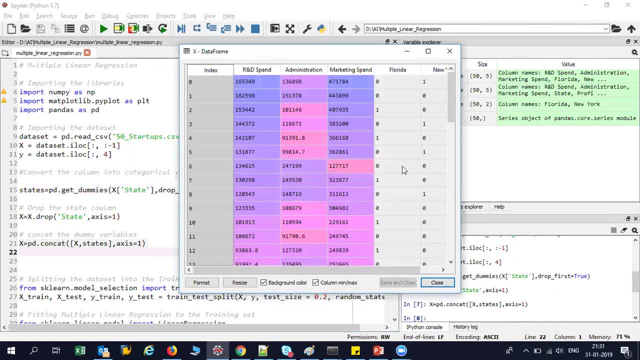 Category features has got converted into two columns and all our integers. Now I can easily access this and this becomes my independent feature. This is the input that I'm going to provide to my model to train it, And you can see over here I'm having R and D spend. 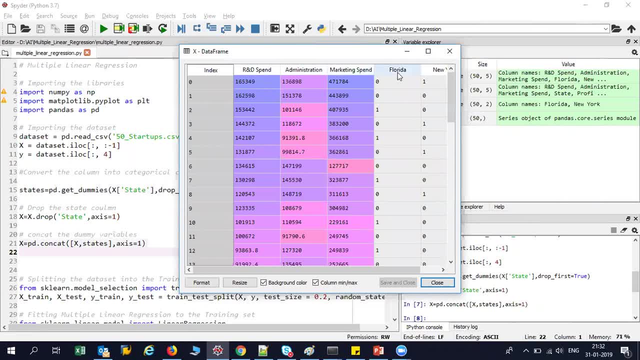 as one feature, administration as another feature, marketing spend as another feature. Florida and New York: Now the same equation. what will happen is that you know how many slopes we will be having now. Now you can see that I'm having my beta one slope over. 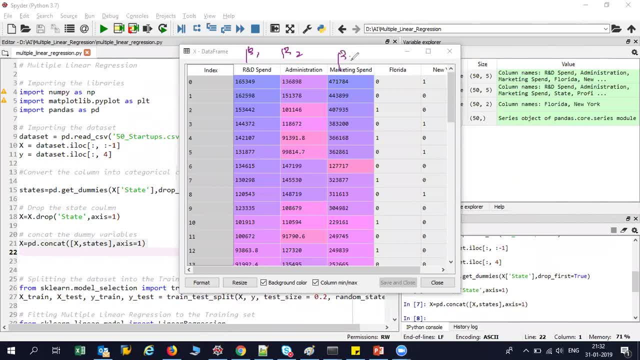 here for R and D spend, Beta two for administration, beta three for marketing, beta four for Florida and beta five for you. So for five different coefficients will be there with that We need to calculate and one intersept which will be beta zero. So all these coefficients has to be calculated. 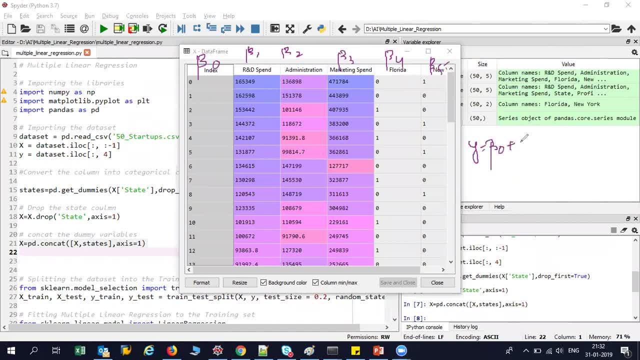 And this is basically given by the question: why is equal to beta zero plus beta one X one plus beta two into X two plus beta three into X three plus beta four into X four plus beta five into X five. Now You've got beta five and two X five. Now, again, you're just. 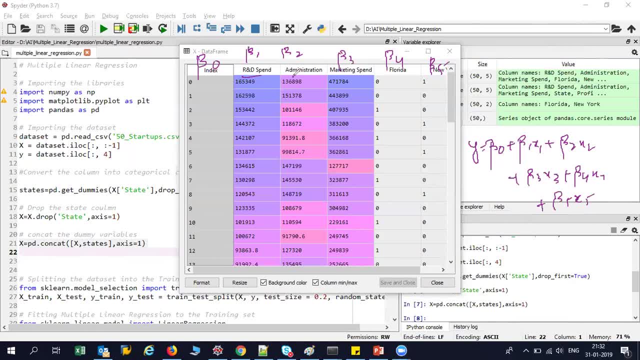 you know that X1 is basically my R&D spend, administration is my X2, marketing spend is my X3, Florida is my X4 and New York is my X5. So this is how my equation gets converted. Now, obviously, if we have multiple independent features, what we can do we have to use multiple. 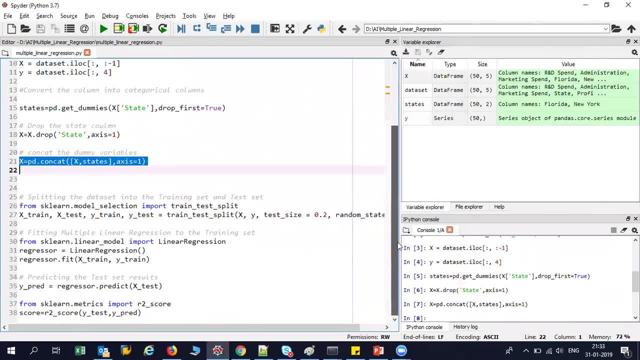 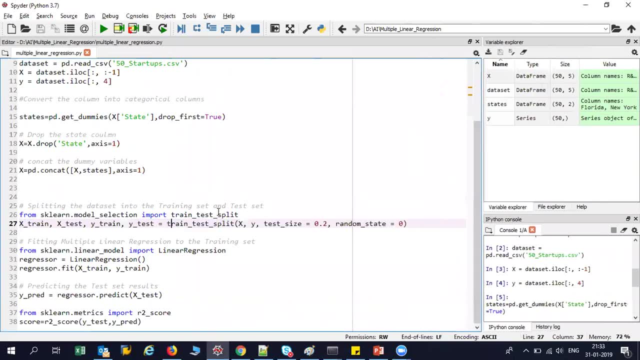 linear regression. Now what I will do is that I will go and do the train test split first of all. Now, in train test split, I am using the library called as train test split. In this I am taking X- Y, my test size is 0.2, my random state is 0 and random state you. 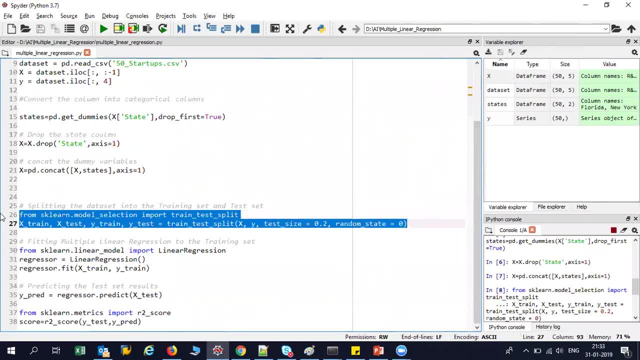 can select any, so that the train test split gets automatically randomly selected. So as soon as I do this, I implement this code. you can see that now I will be creating multiple values like X train, X test, Y train, Y test. So all these values have been created. 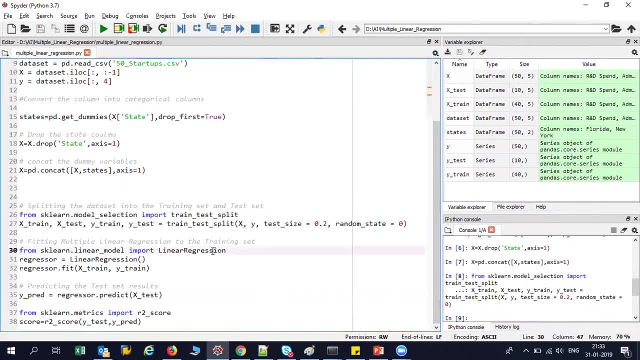 Now what will be my next thing? The next thing is that I am going to create my linear regression model. So as soon as I create this linear regression model, you can see that I am importing from sklearnlinear underscore model. I am importing the linear regression In this linear regression as 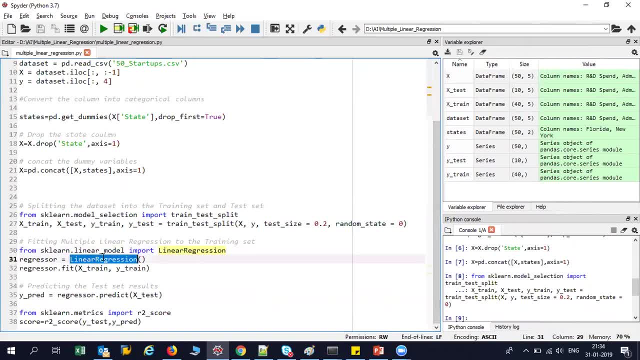 soon as I import it, I have to initialize this object. Now, guys, you may be thinking, is there a different library for multiple linear regression? No, we will be using this linear regression library only. Only our input data will be changing. Now my input data is: 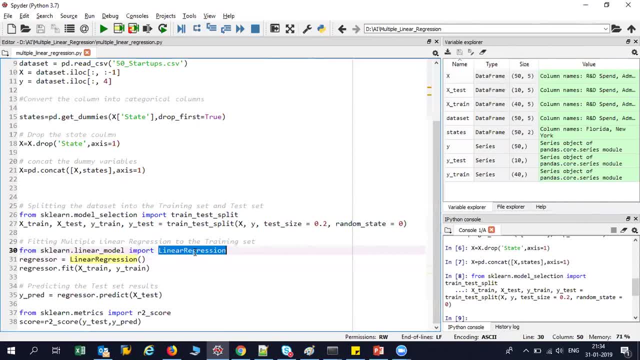 having multiple features. right, In simple language, I am going to create my linear regression model, So I am going to have multiple linear regression. Our input data will just be having one independent feature and one output feature. But now, in this case, if you are considering multiple, 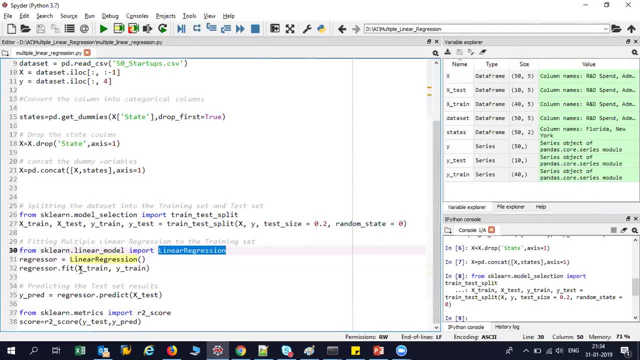 linear regression. it will be having multiple independent features. So now I have over here, I am initializing it with linear regression, I am fitting with X train and Y train. So finally, I will execute this. Now you can see as soon as I execute this, my model will. 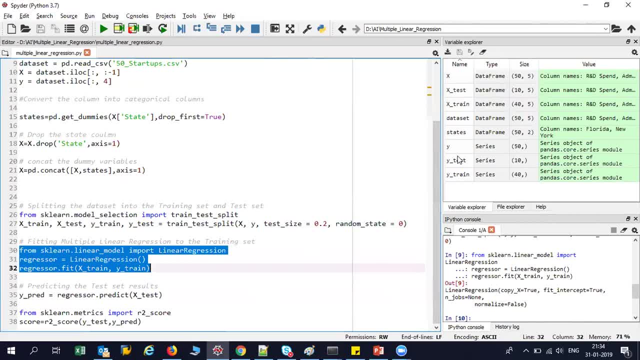 be ready Now. the next thing is that I have my X test data. I am going to do the prediction for the X test data. So I am going to do the prediction for the X test data. So I am going to do the prediction for the X test data. So I am going to do the prediction for the Y test data. So 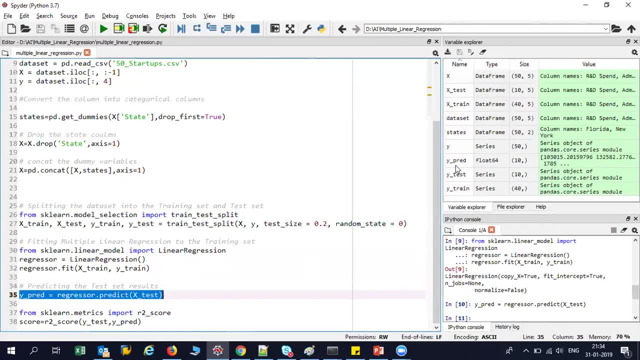 I am going to do the prediction for the X test statement, send it to X three times Cuz. that means when I want to do the prediction for the X test statement I can collect this data. This is my Y cared. Now my Y pred is created right. 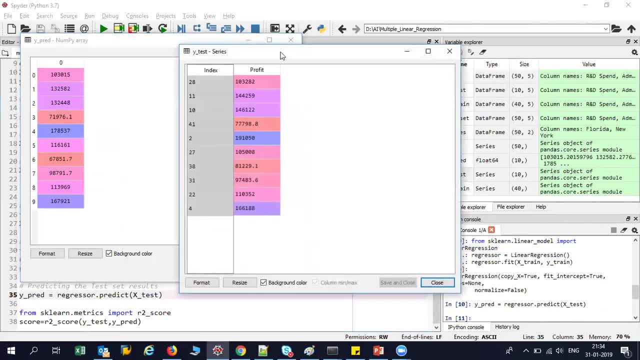 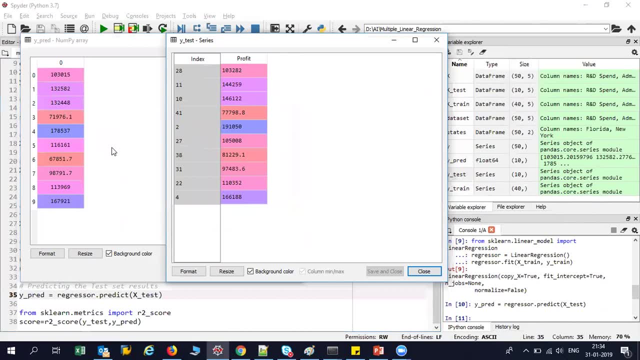 And this is my. Now. my Y test is created. Now the next thing is that I want to compare whether this Y pred and Y test are well and good, or is my accuracy better? Is my accuracy good When compared to the real value that is Y test. For that, what I will. 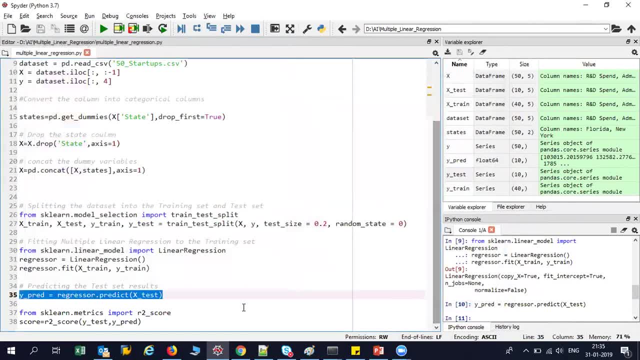 be doing is that I will be implementing a concept which is called as R squared. R squared, R-square, basically, is a concept that I'm going to discuss. okay, R-square formula is basically given by something like this: You can see this: R-square is nothing but. 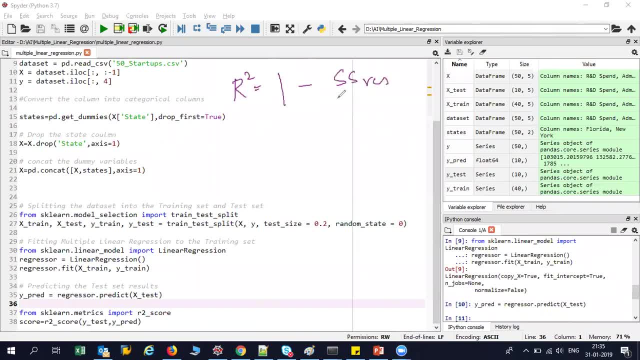 1 minus sum of residual Divided by sum of mean. now when I say sum of residual, sum of residual is basically given by this particular equation: average of I is equal to 1 to n Y hat. y minus y hat y hat is basically my y predicted value, whole square. 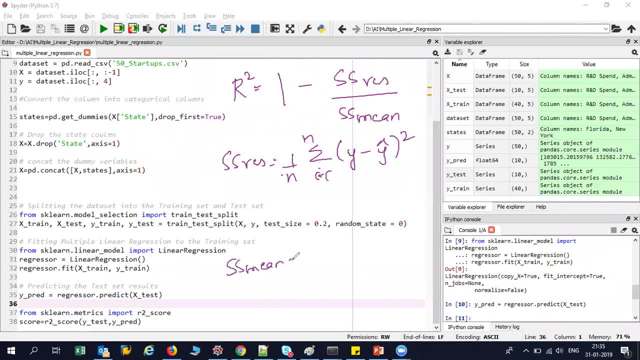 Whereas SS mean is basically given as 1 by n. summation of I is equal to 1 to n. Y minus y mean whole square. so obviously if we We will always know that SS, RES and SS mean from this two if we calculate in this particular way. 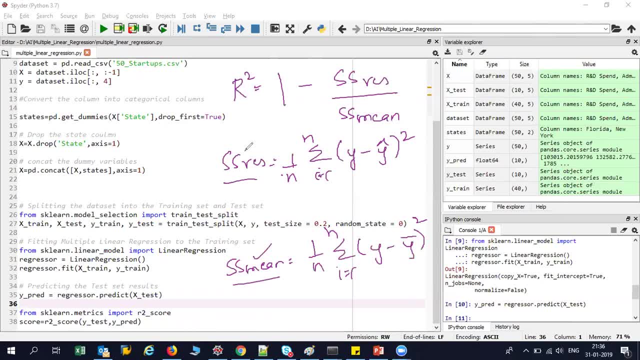 so basically, SS mean will Always be greater than SS RES. So SS mean will always be greater than SS RES if our model is very, very good. So this value that I am doing a division will be a small number. So 1 minus small number will be ranging between 0.8 to 0.98, somewhere around this right. 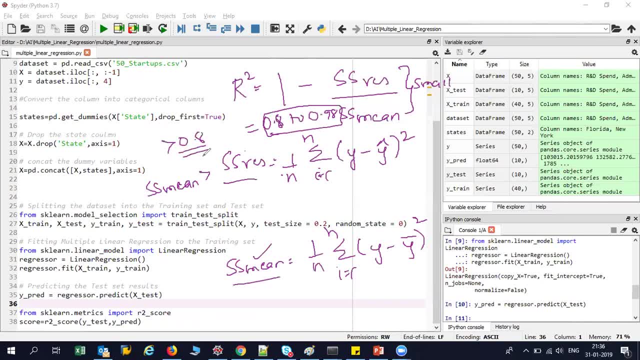 most of the time will be great. getting value greater than 0.8- and usually the R-square values comes between 0 to 1 and More nearer to 1- basically indicate that this model is very, very good, right? So what we'll do is that we'll try to calculate the R-square value, and that is also present in that. 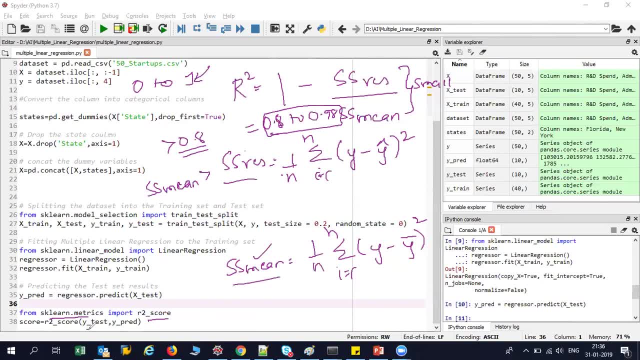 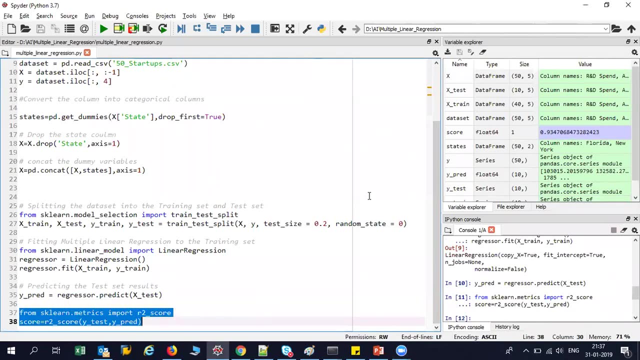 Sklon dot matrix and in the R-square value I just have to give my y underscore test and y underscore prime. So as soon as I give this, you can see that Let me just execute this. if I execute this and If I press shift, enter. now my square value is coming around point. 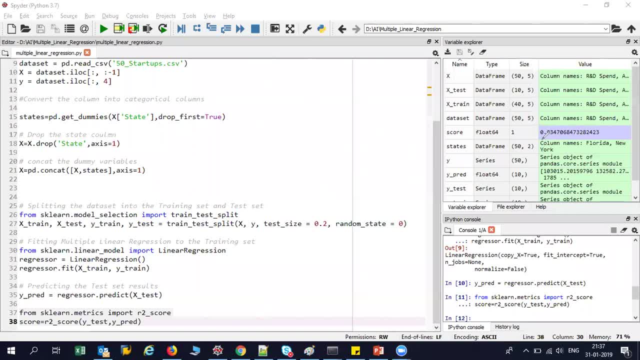 Now, when I see my score value as point nine three, which is very, very nearer to one- point nine Three is nothing but very, very nearer to one- Basically indicates that whatever model we have actually designed over here- It is a good model- Is able to solve this multi full linear regression. 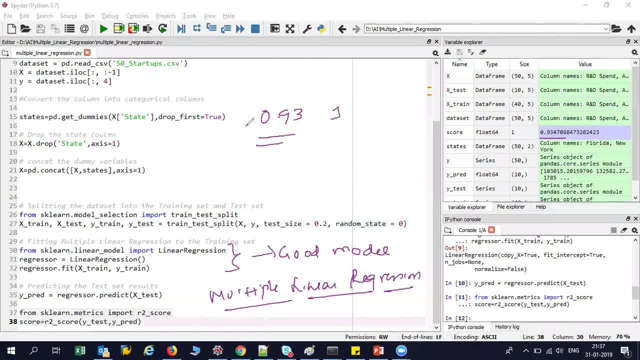 The perfect example of multiple linear regression. I have also got a model where I'm using this R-square values or R-square score to measure how my model has done. So I hope you like this videos, guys. please share with your friends. Please subscribe the channel. Please like this video. 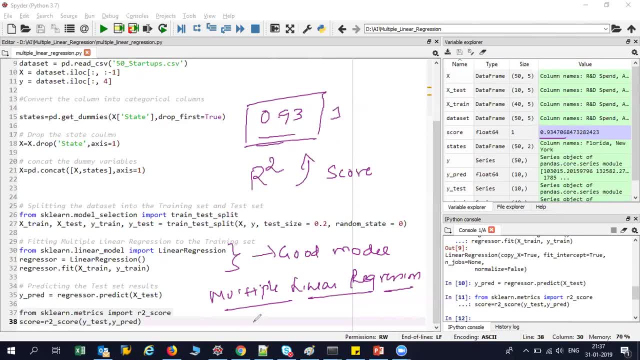 Please let me know, like if you need any more videos, you can put down the comment. You can put down your comments in the comment section, and I'm hoping to cover more different kind of videos. I'm going to start a deep learning playlist, so I hope you like this video, guys, and 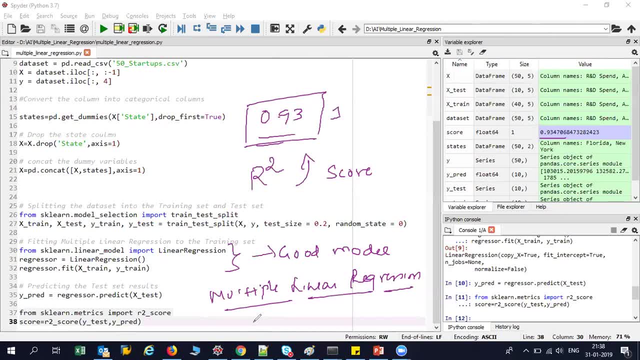 Please Keep on always learning. Please make your best efforts to learn more and more things and try to help others. So I'll see you all in the next video. Happy learning guys. Thank you one and all. Thank you one and all, and I'll see you in the next video. Thank you.